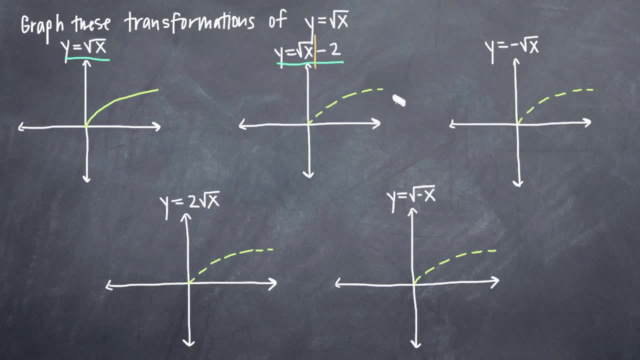 up or down within the same set of x values. What we mean by that is that we have the function y equals square root of x minus 2.. Every point that would be on our original graph y equals the square root of x, is just going to get moved down two units. In other words, we're 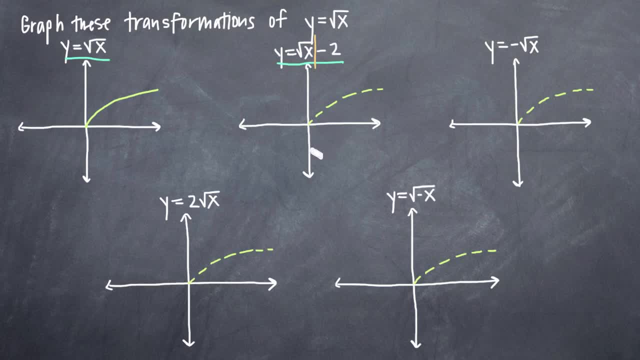 going to take every point and shift it down by negative 2.. That means that let's say it's about here. We'll take every point and shift it down by negative 2 so that our transformation actually looks like that. In this third example here, where we have y equals negative square root of x, we have 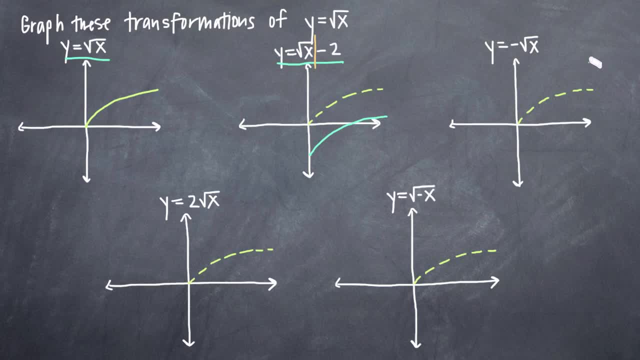 notice a negative 1 multiplied by our square root of x term. Whenever you have a constant multiplied by your original function, that means you're either going to be stretching or shrinking your graph and or flipping the graph across an axis, In this case, every. 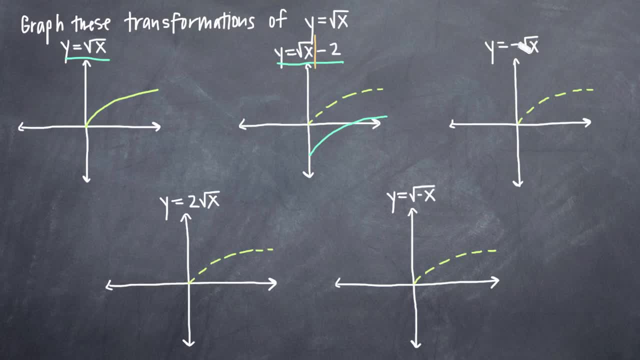 point over x is going to return a certain y value. But this time, now that we've multiplied by this negative out in front, we're going to get the same y value, but multiplied by negative 1.. So this is just a transformation flipped across the x axis and the graph looks: 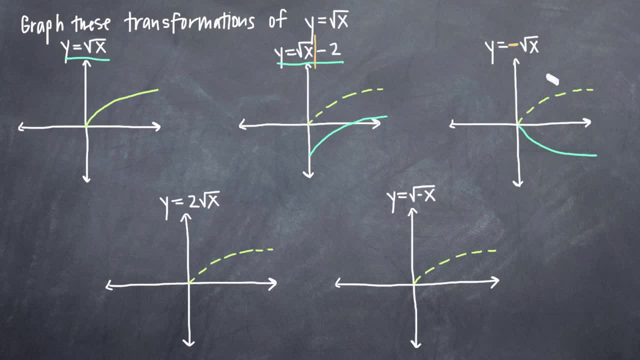 like this. So just remember that if you've got your original function square root of x with a negative out in front, that means you're going to be flipping it over the x axis. Similarly, here with our next function, we're going to get the same y value but multiplied by negative. 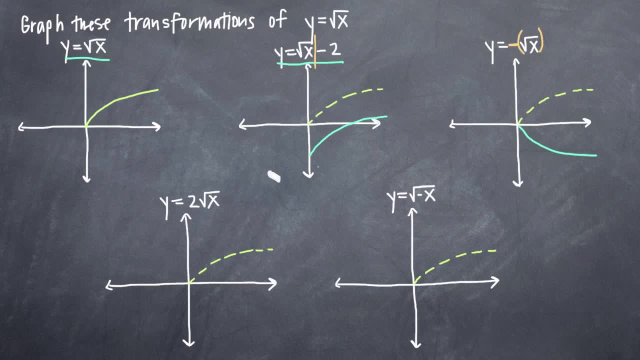 1.. This is just a transformation flipped across the x axis and the graph looks like this: We have a constant coefficient multiplied by our original function. Same with the last one. we have negative 1 multiplied by our original function. Now we have 2 multiplied. 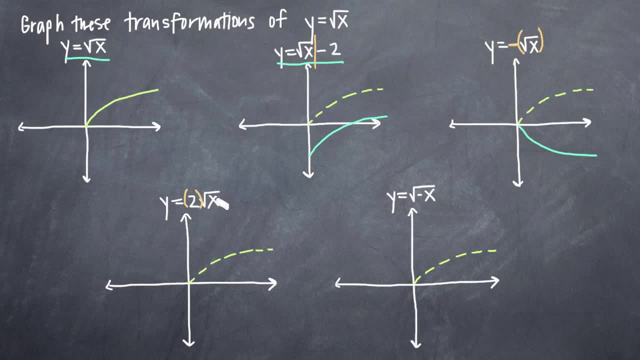 by our original function, And what that means is we're going to be stretching the graph by a factor of 2. So when we draw the graph, instead of every y coordinate lying along the original function, the new y coordinate will be double what the old one was, So that'll 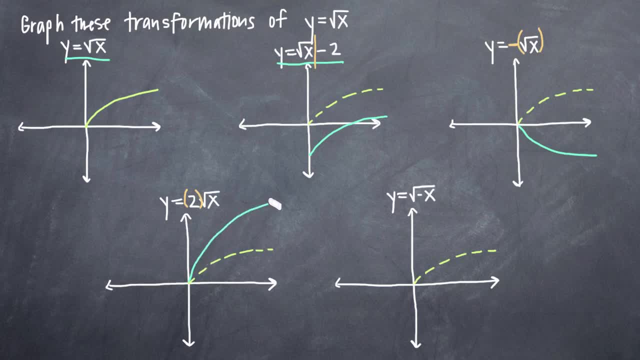 look something like this, And the way you can think about it is: we would have had our original y-coordinate here. Let's say that that's at 1.. Well, our new y-coordinate will be double that a factor of 2, so the new y-coordinate will 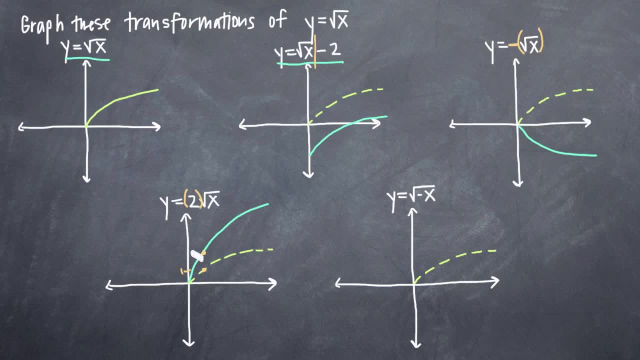 be here at 2.. Same thing here: if our y-coordinate was 3, our new y-coordinate is 6.. So it just stretches the graph by a factor of 2.. Think about it this way: if we had had negative 2, if we had had y equals negative 2 times. 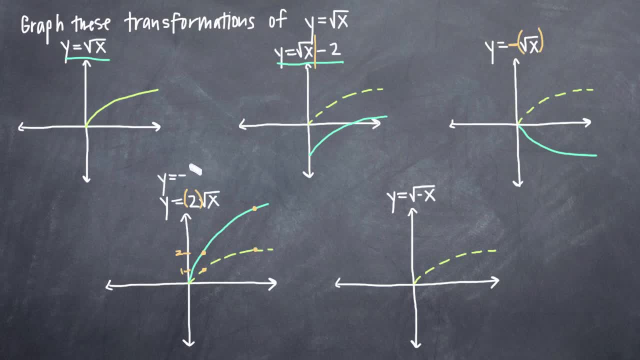 the square root of x. we would have been stretching the graph a factor of negative 2 and flipping it across the x-axis, and that would have looked like this: Keep in mind that the same thing goes for shrinking the graph. if we had the function, 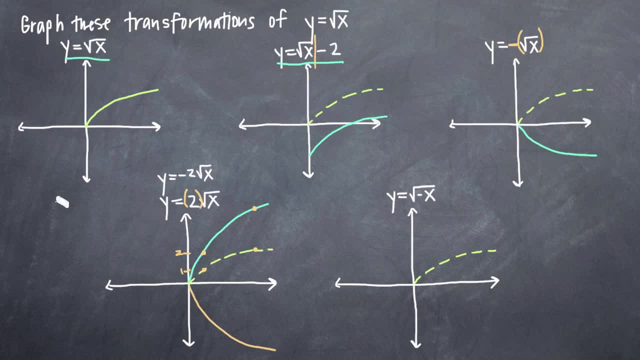 y-to-x-to-y-to-y-to-y-to-y-to-y-to-y-to-y-to-y-to-y. Okay, So y equals 1, half square root of x. We're dividing our original function by 2 instead of multiplying it by 2, and that would 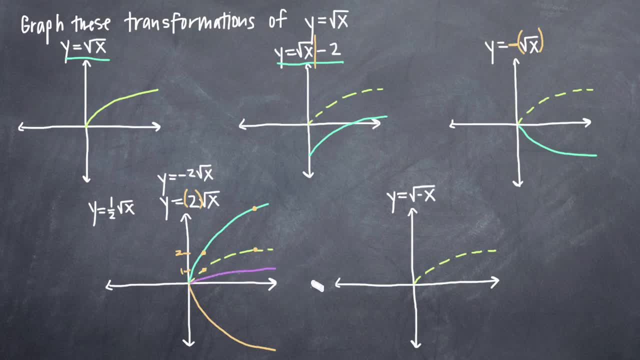 have looked something like this, So I hope that gives you an idea of the transformations you'll see when you have a constant coefficient multiplied by your original function. In the last graph we have: y equals the square root of negative x, and this one here is similar. 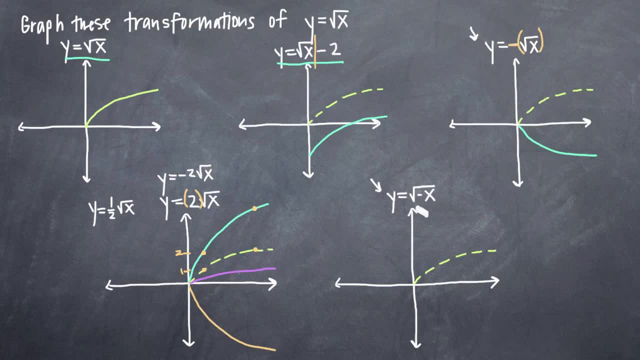 to this graph that we did, in the sense that all we've done is add a negative sign, except that here we've added it in a different place. It's inside our square root sign instead of outside our square root sign. Remember that before, the negative outside of the square root sign meant that we were 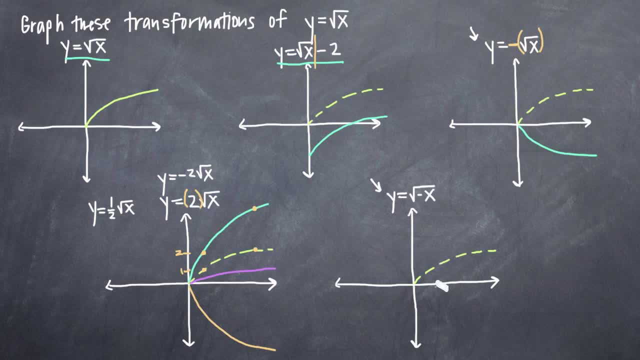 flipping across the x-axis. Since we have a negative inside our square root sign, that means we're going to be flipping across the y-axis. So our graph is going to look like this and that makes sense, because when we have a negative sign inside our square root here, 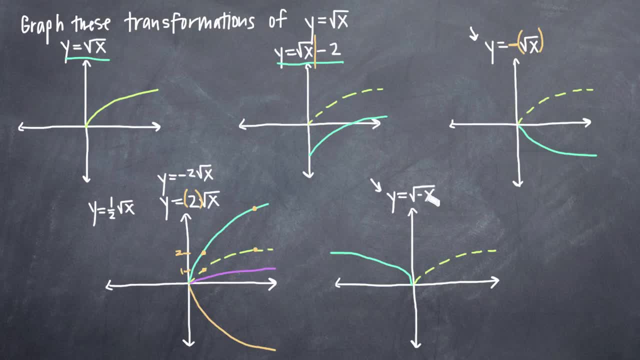 We know right off the bat that we can only have a positive value underneath our square root. In order to get a positive value underneath the square root, that means we're going to need to put in a negative value for x, so that, for example, if we plug in a negative 2, we'll 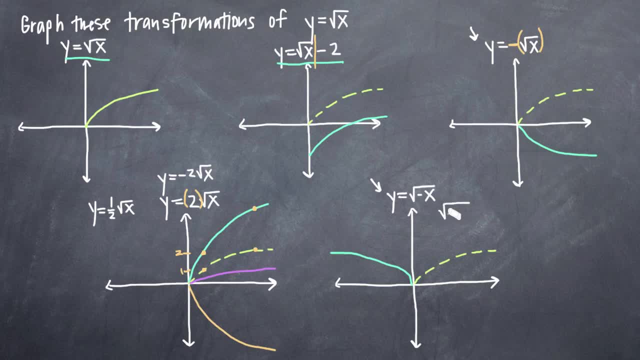 get the square root of negative negative 2, which will equal the square root of positive 2.. The only way to get a positive value underneath the square root sign is to insert a negative value for x, which will equal the square root of positive 2.. 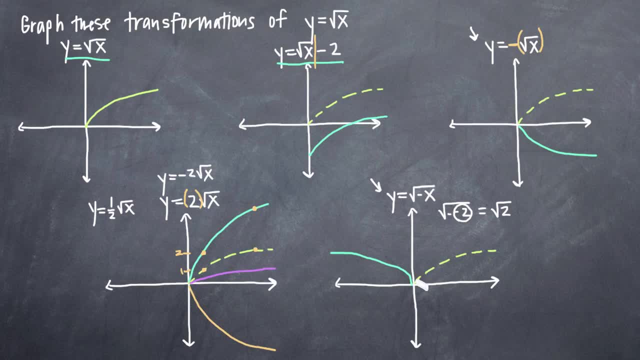 Okay, So that's it. That's a preview into some basic transformations, So I hope you found that video helpful. If you did like this video down below and subscribe to be notified of future videos. I'll see you in the next one.